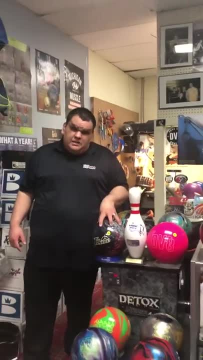 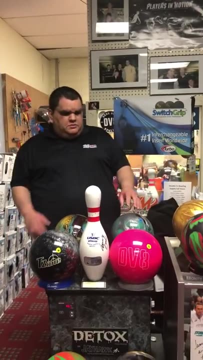 Here we have a couple options. We've got a nine-pound ball here, a 10-pound ball here, We've got a 12-pound ball and we've got 14, and then we've even got 15s here. So the biggest thing you want to look at is the more weight you have, the better. 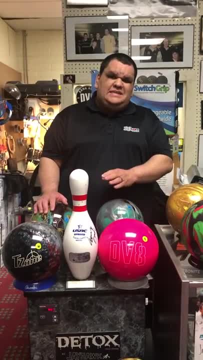 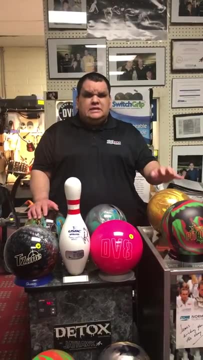 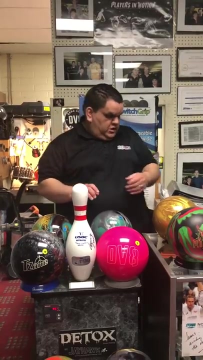 And when it comes to weight blocks, if you go from a 10 to 12-pound and 13, to a 14-pound bowling ball, the weight block in these reactive balls is not going to be the same. It's going to be a, let's say, about half the size of an actual weight block that's in a bowling ball. 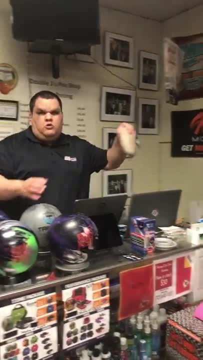 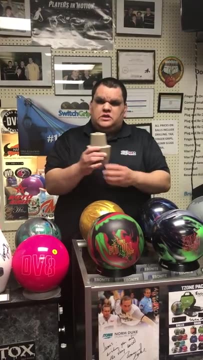 So just to give you a for instance, this here is a whole weight block. So if you get a ball, that's about 10 to 13 pounds, think about it being half this size. The reason being is a weight block typically weighs six to eight pounds inside of a bowling ball. 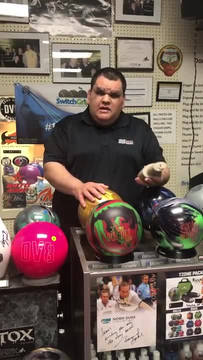 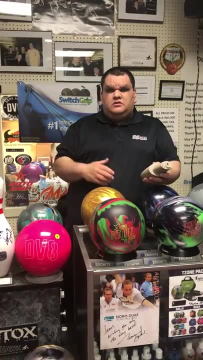 So when you have a 14-pound bowling ball they have 14,, 15, and 16s, have about the same weight block size and weight which is key In 10 to 13,. they're not going to have that much weight block inside. 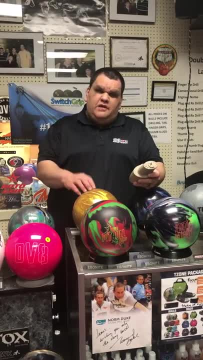 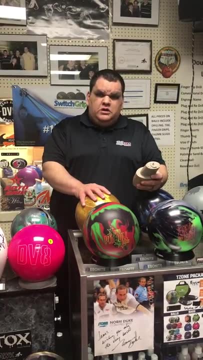 because there's so much core material on the inside and then cover stock that you have to have inside of a bowling ball. So that's really key when it comes to bowling balls and weight, especially for those of you who are going to buy reactive balls. 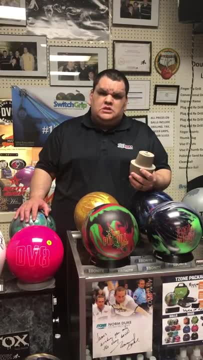 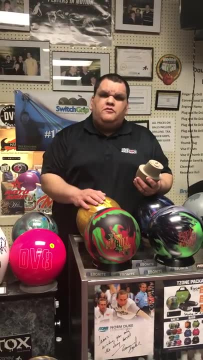 It's really important to be able to throw and handle about as much weight as you can physically, And that's the thing. I get a lot of new bowlers that come in here and I always tell them: look, if you've bowled before, it's like riding a bike. 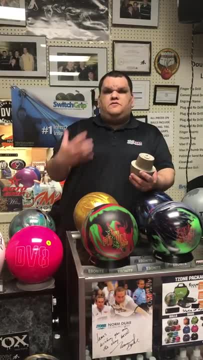 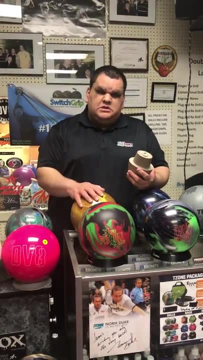 If you haven't bowled before, you can learn great muscle memory. Obviously, the fit's going to be important. That's going to play a key role into not injuring yourself and having fun on the lanes and being able to throw more weight, which when you throw more weight in a bowling ball. 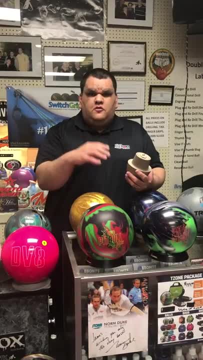 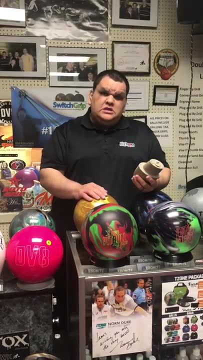 that gives the ball more potential to hit down more pins, therefore get more strikes and in turn higher your average, So that way you're not having to shoot so many spares. So just to give you guys an idea and tip on weight: 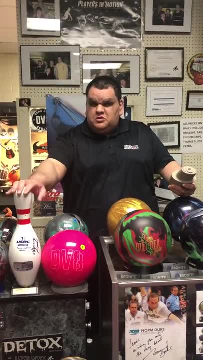 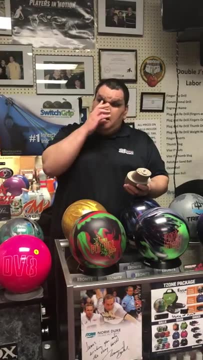 remember a bowling pin: 3 pounds, 6 ounces, so 36 pounds of pins. for every pin back there, That's 10 of them. Then you've got all different weights of balls. So when you're looking at getting a bowling ball, I would suggest when you come in here,